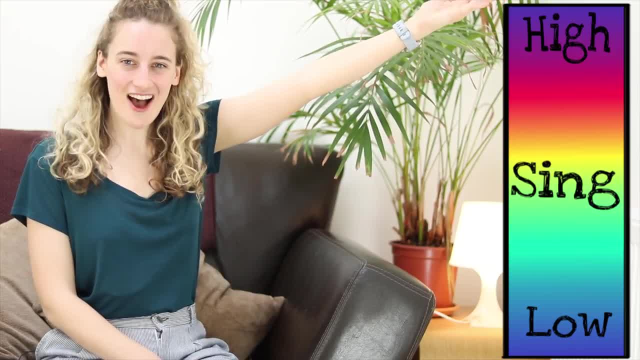 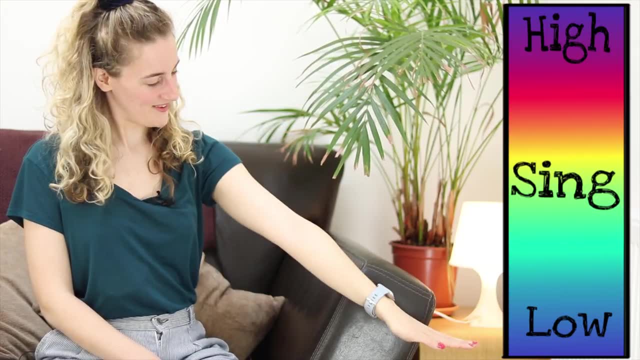 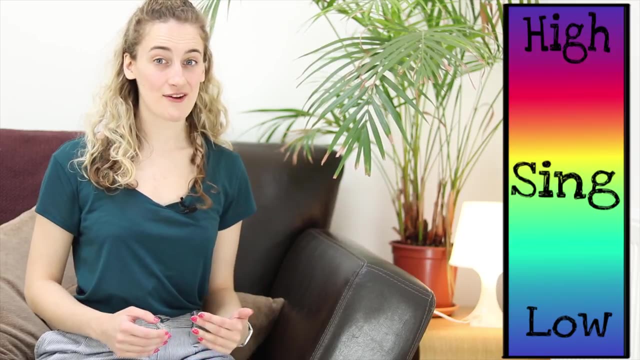 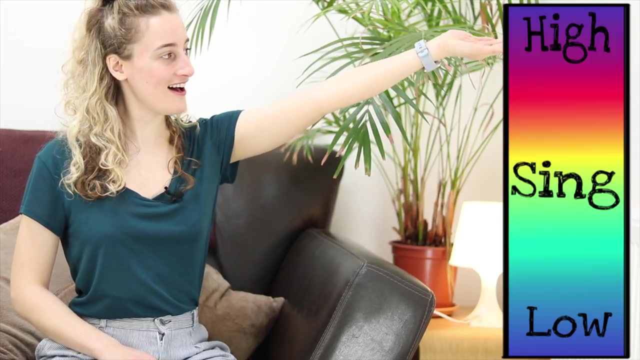 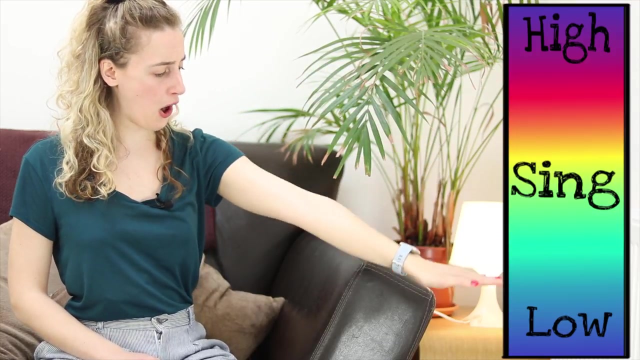 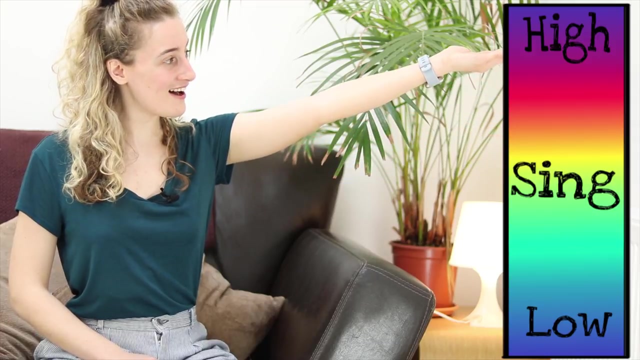 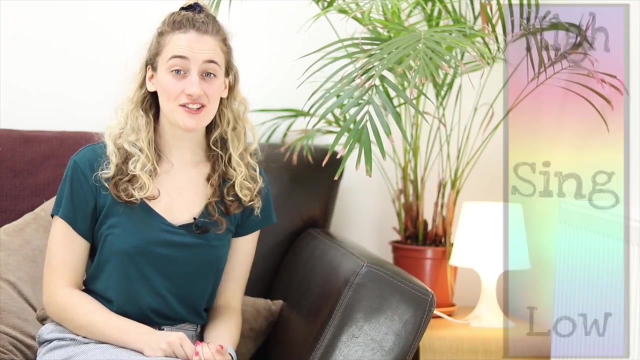 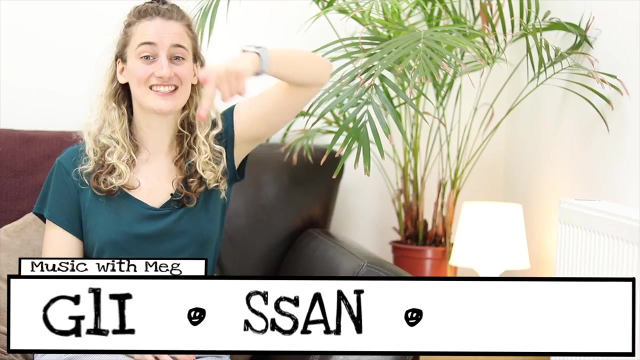 High, Low, High Low. Now can we go from our lowest note to our highest note without stopping? Follow me. Good, and now back down One more time. Here we go And back down. Musicians call this a glissando. Repeat after me Gli-san-do. 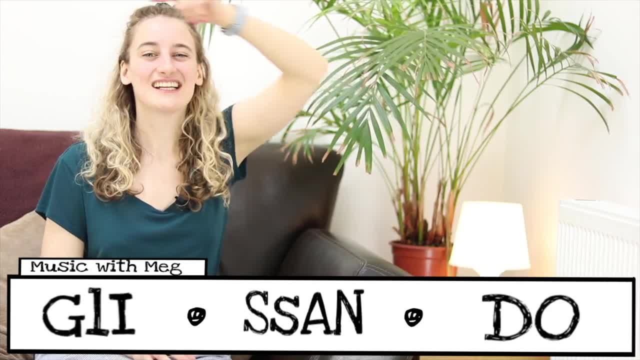 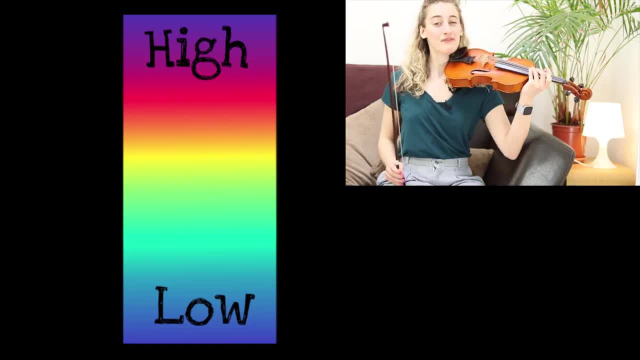 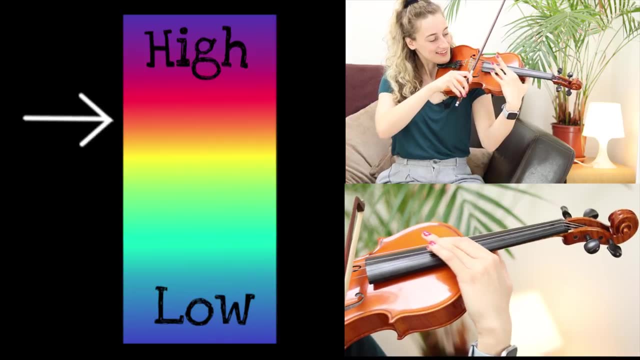 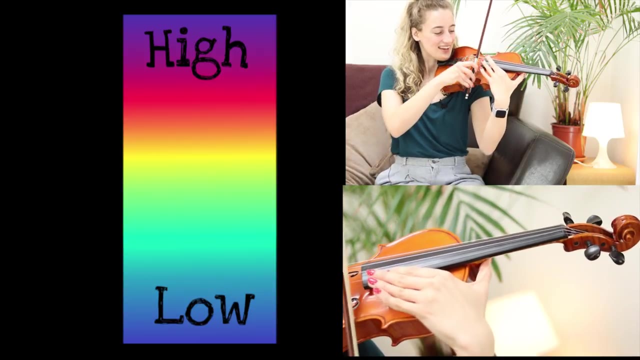 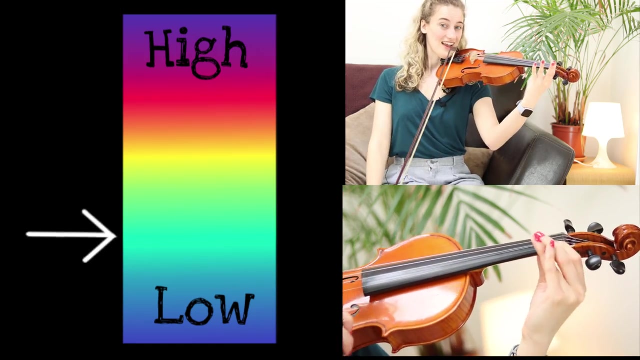 Gli-san-do, Glissando. Now let's do some glissando With my violin. Let's go from low to high And back down, And a bit faster. One more time. Different instruments have different pitches. Let's have a listen to the highest pitch. 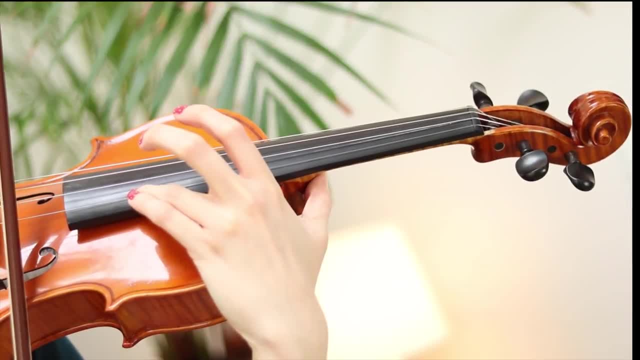 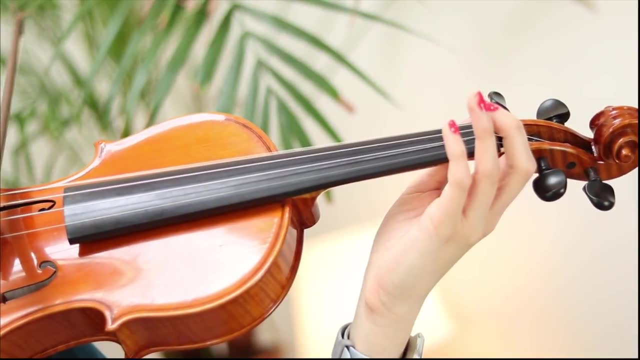 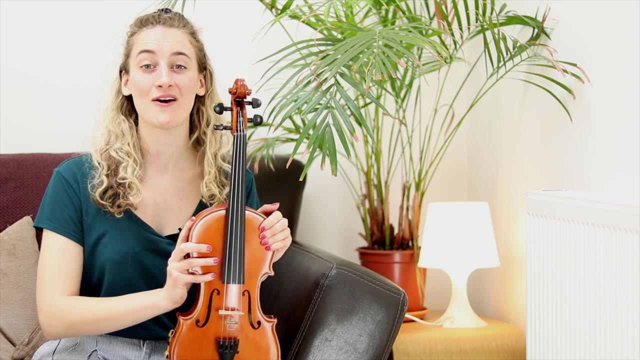 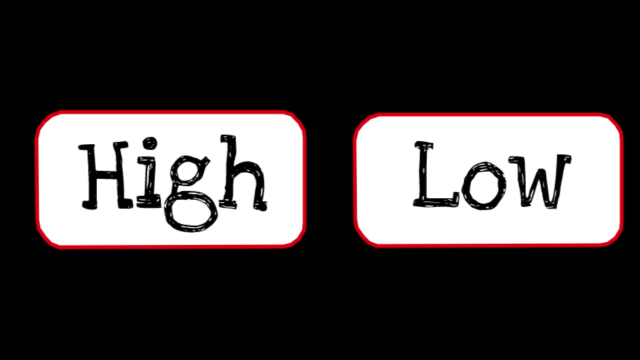 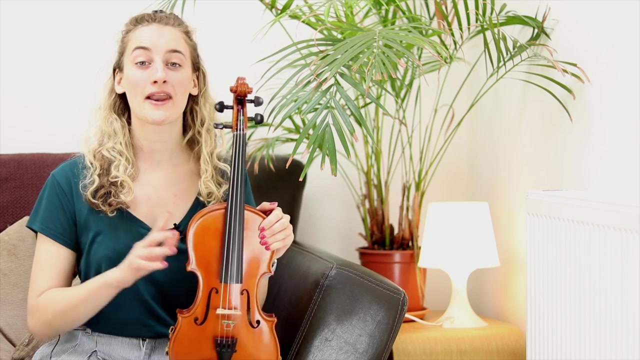 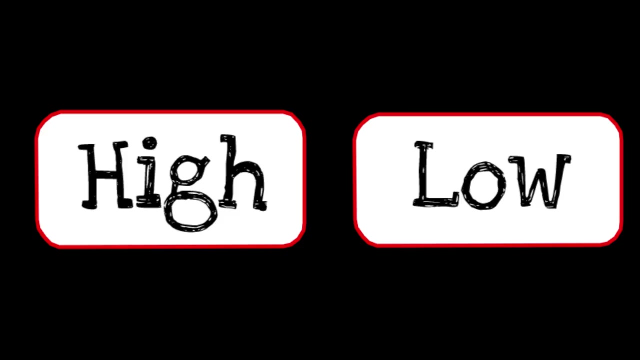 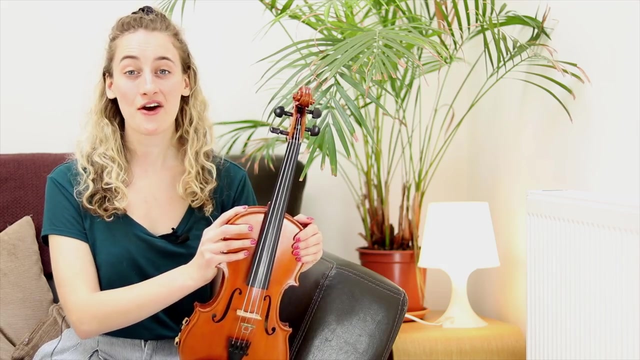 highest note my violin can play, And now let's listen to its lowest note. Now have a listen to this note. Tell me, is this a high note or a low note? High or low, High? And how about this note? Is this one high or low? High or low, Low? How about this note Tell? 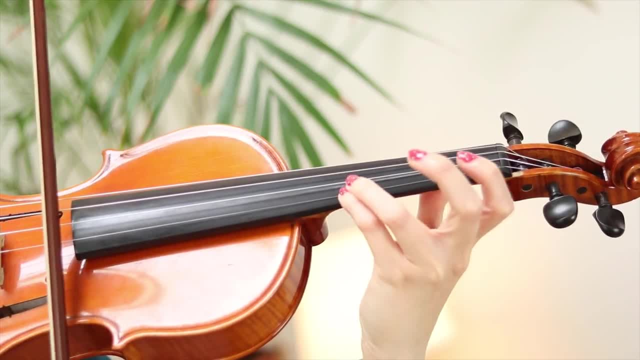 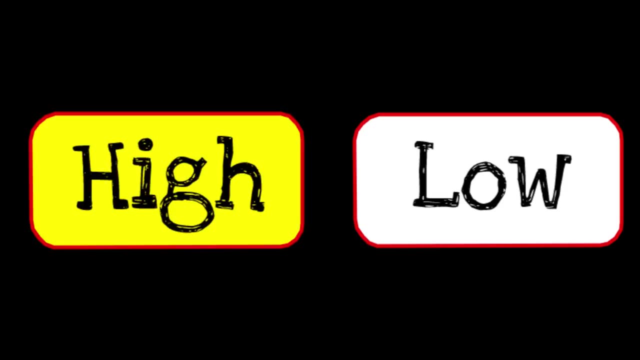 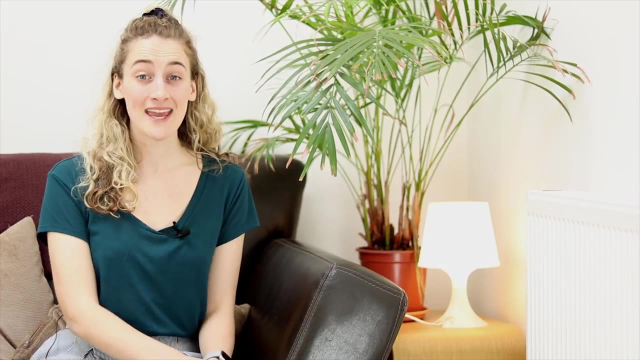 me? is it high or low? High or low High, Just like that. And now let's listen to this one. How about this note? Is this one high or low? High or low High? And how about this? one Date is different, but in a few ways they can be very different. Let's look at. 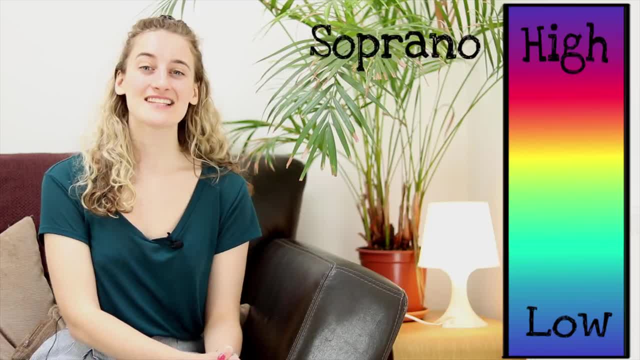 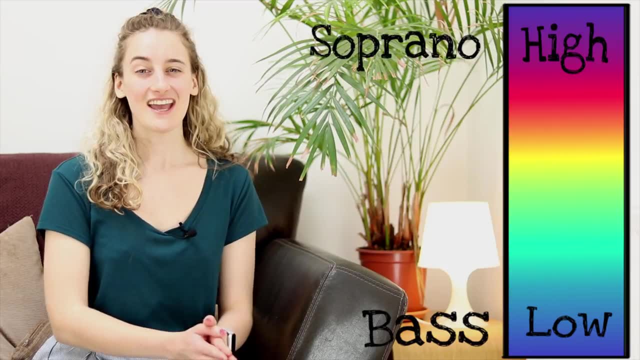 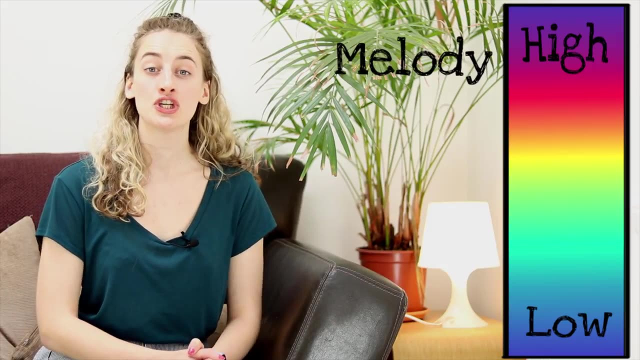 this note on an instrument for a demonstration, For example, Sit. Just like musical instruments, different people's voices have different pitches. So a soprano singer has a high-pitched voice and a bass singer has a low-pitched voice. In music often instruments and voices with